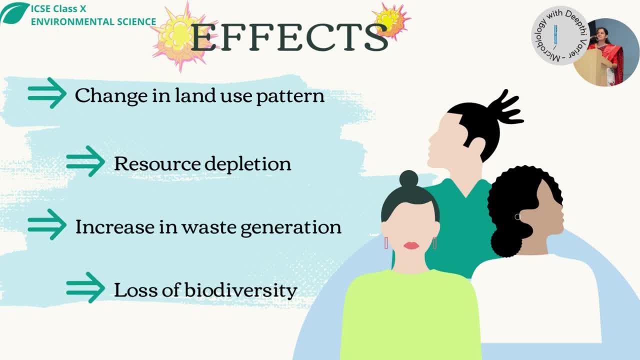 for those individuals to get food. So there has been a shift from forest ecosystem to more of urban ecosystems or people, you know, living in the rural areas. All of this has this land use pattern has shifted from the natural forest ecosystems to urban or settlements where 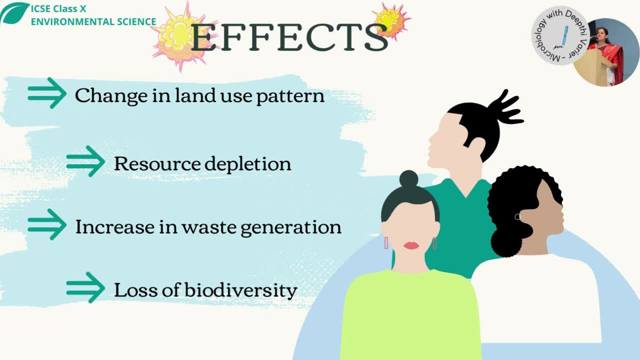 people are living or where they are working. So that is the biggest change that has happened and that is a big problem when we look at the global scenario. We have also had resource depletion. It's not just the land resource which has been which is being depleted, Many other resources also. 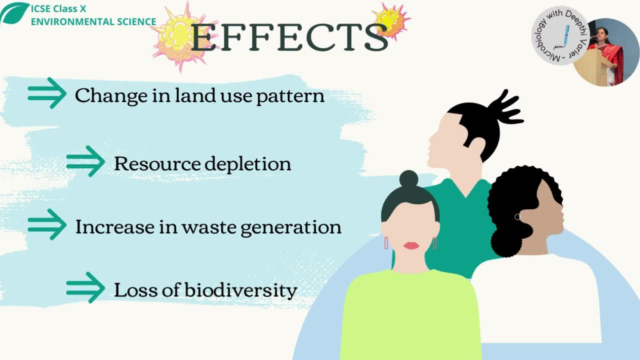 have reduced, like food, the shelter problems are there, healthcare is a big trouble. Electricity is a big problem in several cities and you know rural areas. Many of the forests have been converted into croplands, So resources are coming down quickly. That is resource depletion. 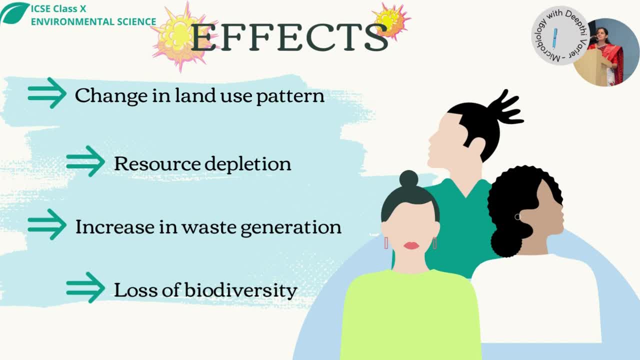 There has been increase in waste generation. This we have seen in a different chapter as well. Waste is one of the biggest problems of society, So as the population increases, so does the generation of waste And, lastly, due to the resource depletion. 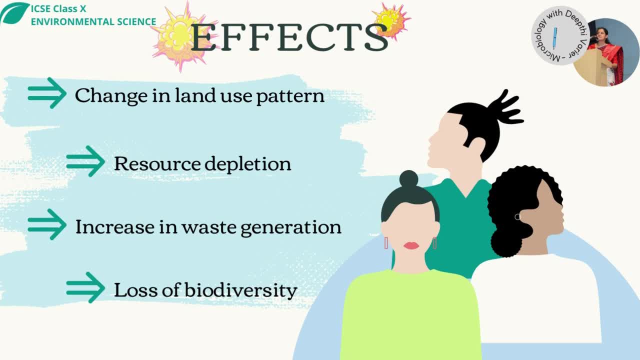 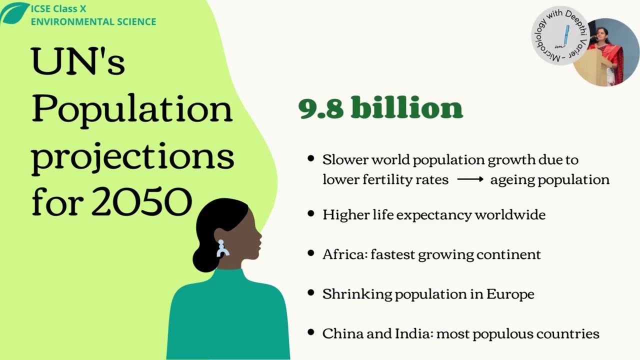 due to the change in the land use pattern, we have had severe loss of biodiversity. So these these are some of the negative effects of the population on the environment. Now, the UN's population projections for 2050 is that the population on earth will reach 9.8 billion. 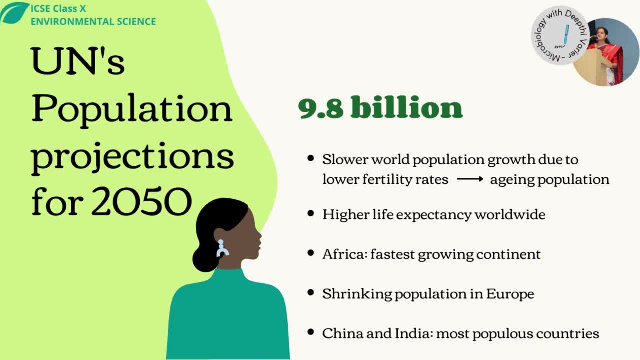 Currently, that is, as of November 15, 2022, we reached 8 billion mark And by 2050, we will reach 9.8 billion. In fact, by 2037, in another 15 years time- we will reach 9 billion. 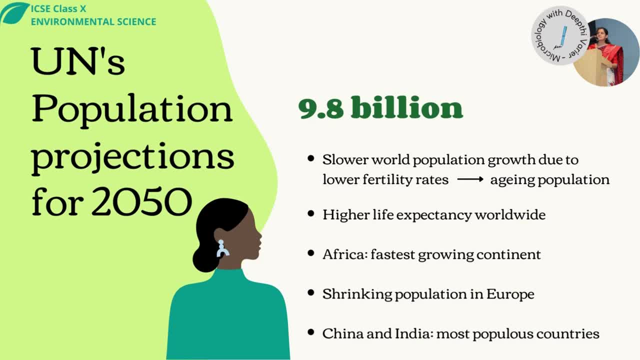 So on the whole, if you see, the population growth has decreased, that is, the fertility rates have come down. due to the fertility rates coming down, the world population is growing at a slower rate, but then that has also led to an aging population, So the number of old people, that is, people who are 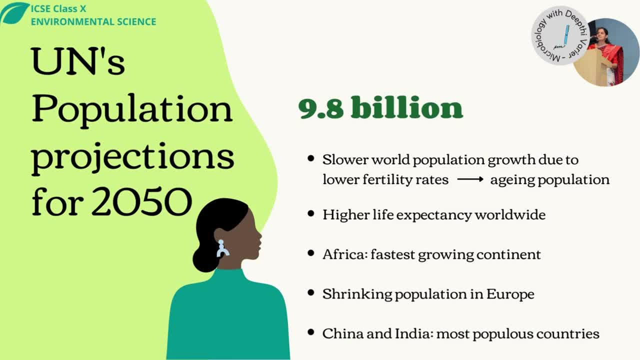 65 and above will be more in the future. Not only that, this report also says. the UN's population projections also say that the life expectancy is higher, So the number of people who are 65 and worldwide, so the global life expectancy, will reach 76 years by 2050 and between 2095 to 2100. 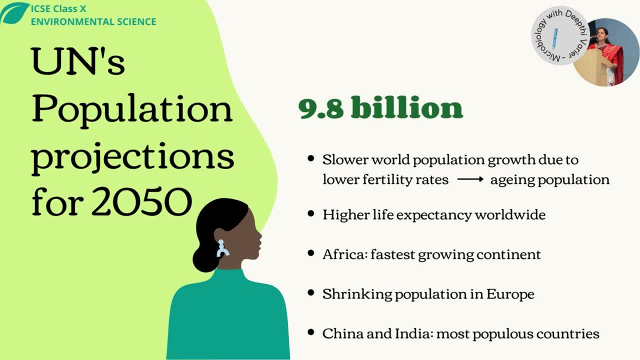 the life expectancy will be 82 years, that is, an average person will live for 82 years by that time, so the life expectancy will go higher and higher. it's already increasing and will further go higher. it also predicts that africa is the fastest growing continent, so developing countries. 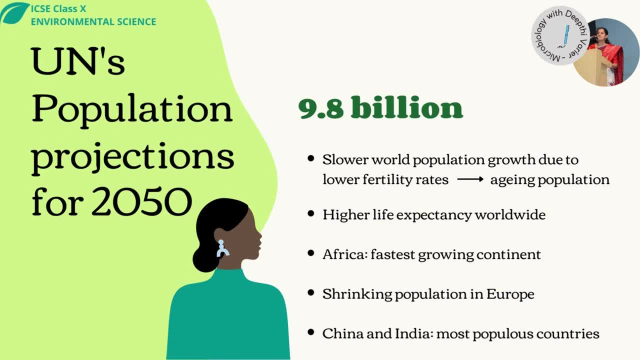 especially in africa, are growing very rapidly, like nigeria, niger, congo, ethiopia, uganda, one of the main reasons being their high fertility rates. that is why these content, these countries in african continent, are growing very fast. the population of 61 countries is expected to. 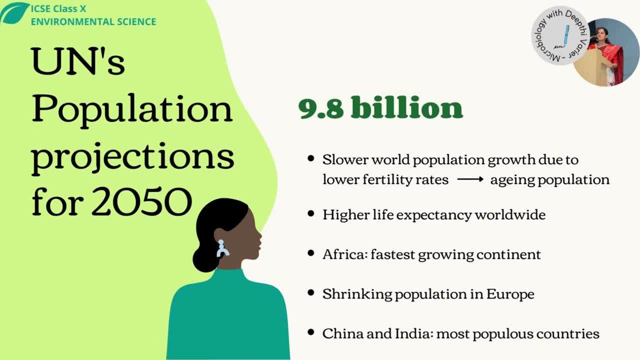 decrease by 2050, and this includes many of the european countries. this is mainly because the fertility is very low and it is much lesser than the replacement level. replacement level is the level that is going to decrease by 2050, and this is the level that is going to decrease by 2050. 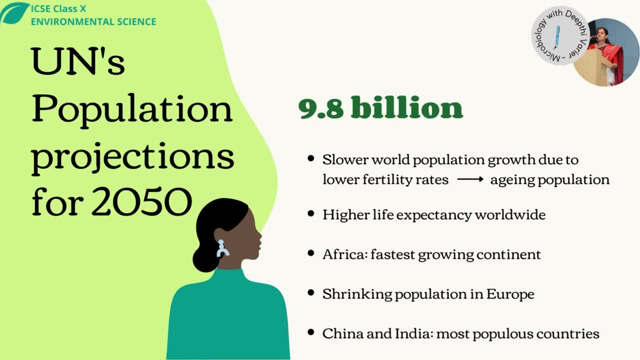 that is required to bring back the population to the original level. so because the number of children who are being born, the birth rate, is much low. that is one of the reasons why the population is shrinking in many countries, especially in the european continent. we also have china and india. 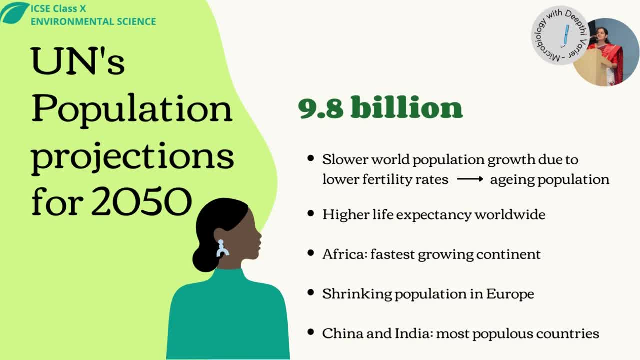 which are the most populous countries, and it says that india will soon be more in population than china. so china and india are already above 1 billion, but they the scenario that is predicted that india will surpass china in population numbers. there are many large developing countries where the average number of children per woman has decreased rapidly, so that is happening. we are. 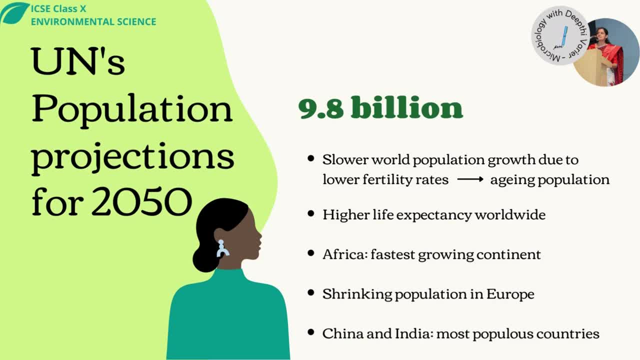 having lesser number of children being born per woman. this is mainly seen in south africa, in iran, in china, in brazil, even in india, but on the whole, if you see we are, india is having more than 1 billion population and it is only going to increase more if certain strategies are not. 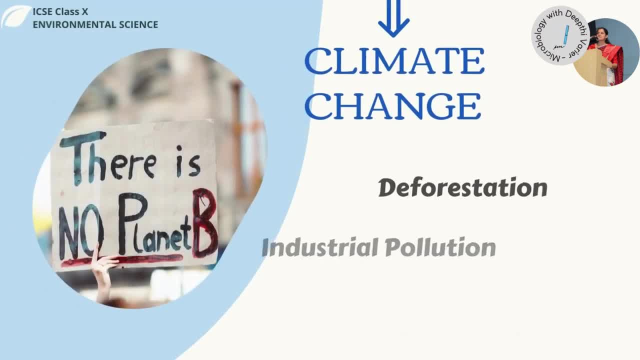 employed or if certain strategies are not put in place. so now all of this has led to the climate change, now the increasing population, or the population growth. not only has it affected the environment, but it has also caused change in the climate pattern, because there is more need for food. 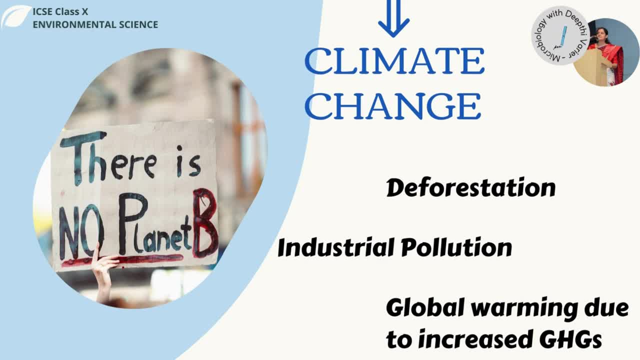 there is more fuel requirement, there is more need for shelter, so that has led to deforestation. deforestation is where the forests are cut down for converting into a settlement or into an agricultural land or a cropland. so forests regulate the temperature. we know that forests are. 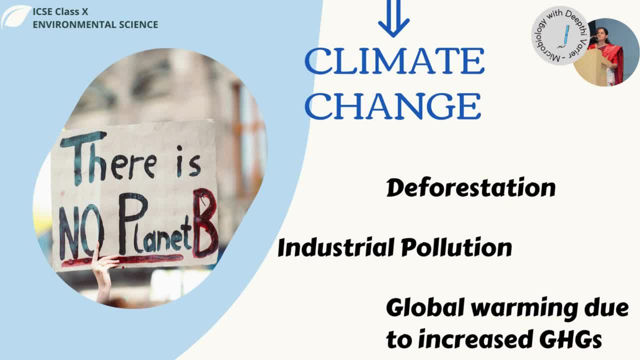 regulating the rainfall on earth and because of the rampant deforestation that has also led to global warming. so global warming due to the increased greenhouse gases, because more fuel is being burnt, that has led to more global warming. it has led to the industrial pollution. so we can 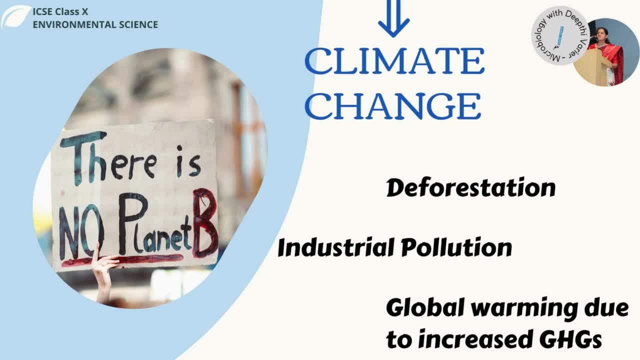 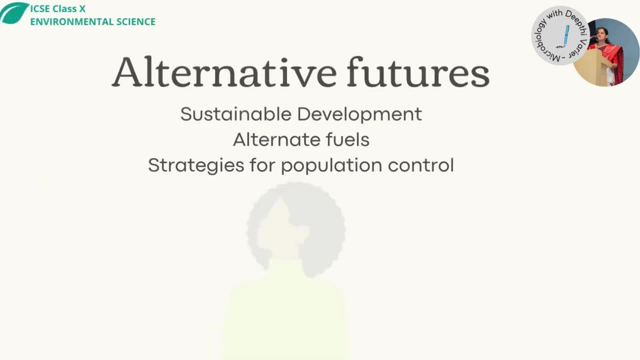 say the population growth has. you know directly it has. it is having a direct link with the industrial pollution because there is more demand for the consumer products. so if you see over here, increasing population does have a very negative and a direct effect not only on the environment but also on the climate. so there are certain alternatives. 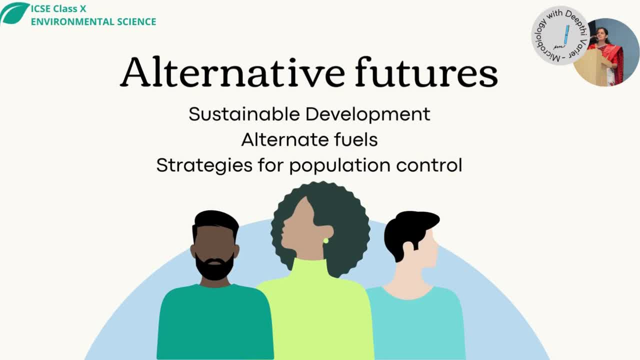 that we can have. we can choose an alternative future if we are able to achieve the low projections that have been given by un. so un has projected in three different variants. they have given a low projection of the population, a medium projection and a high projection if we are able. 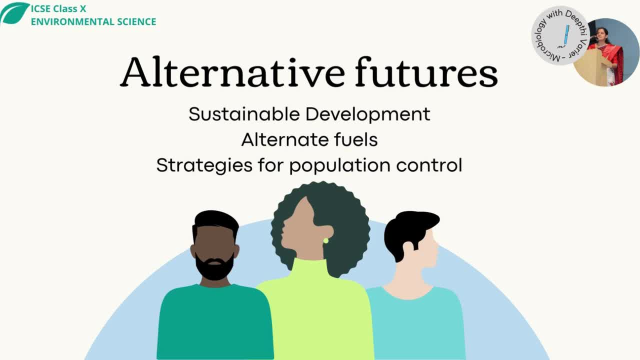 to achieve the low projection of the population that has been given by un, then we will be, you know, having an alternate future. we will be able to control a lot of the negative effects. we will be able to reduce the degradation of the environment. we will be able to reduce the amount of climate change, provided we put in place. 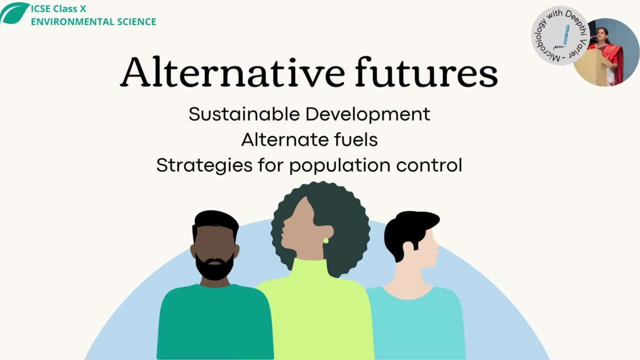 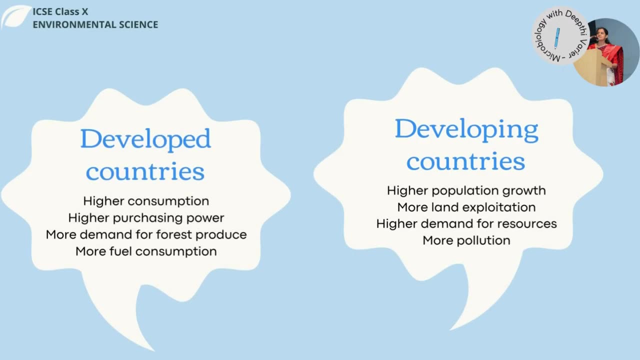 all those strategies. so the alternative futures can be or is possible by sustainable development, by use of the alternate fuels or by implementing the strategies for population control which we will be seeing in the next few slides. now, when we see the developing countries and the developed countries, there is a continuous divide on environmental issues, on development. all of these are, you know. 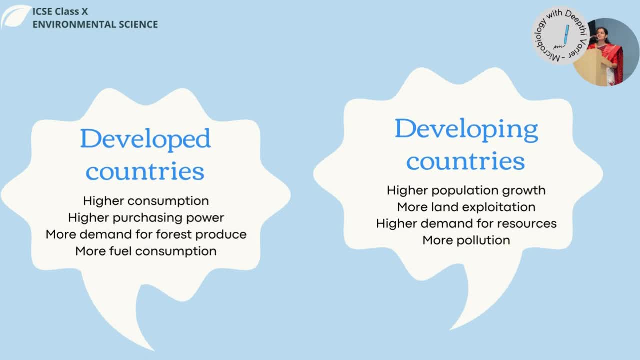 there is a big demarcation between the developed countries and the developing countries. developed countries have more consumption, so every thousand individuals is in a developed country are consuming three to four percent of the earth's resources, in comparison to 9 000 individuals of the developing. 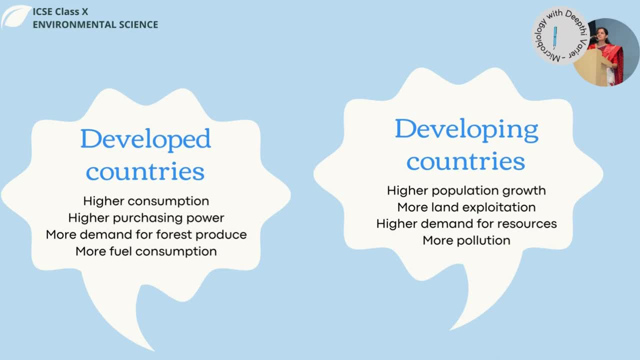 countries. so because developed countries have more purchasing power, they have more consumption. their demand for forest products is much, much more. their forest fuel resource consumption is more. so they do have more consumption because of their higher purchasing power. that is one side of the developed countries. the developing countries are definitely having much more. 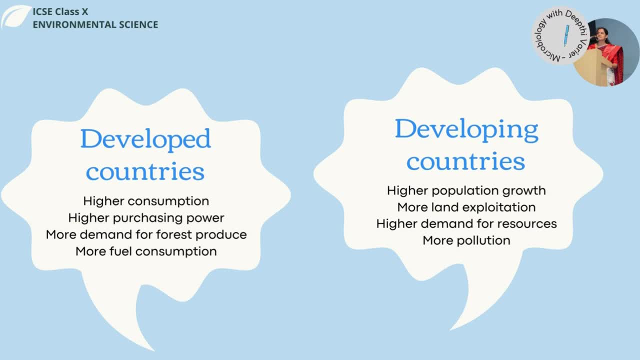 population growth in comparison to the developed countries. and when there is more population growth, automatically there is more pressure on all the sectors to increase their output. so there's more demand for resources, there is higher pollution, there is, you know, more food requirement, which again leads to land exploitation. so these are the different sides of the developed countries. 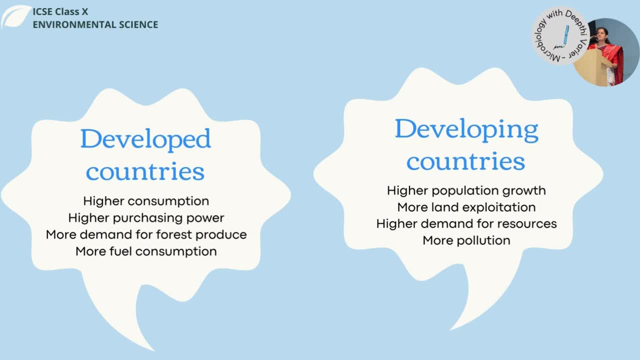 and the developing countries. and due to this difference, due to this divide, there has always been a- you know, a debate on who should be taking more care, who should be putting in more strategies. is it the developed countries or the developing countries? both have each other to blame, so we need 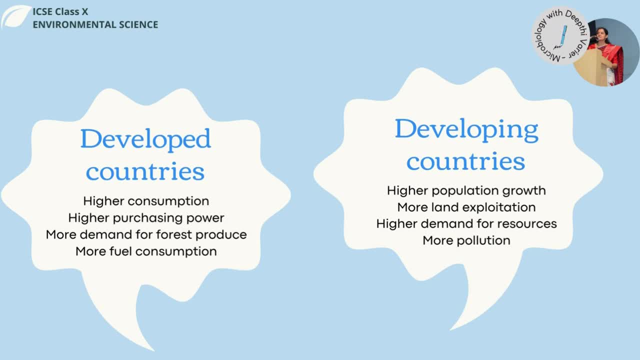 to see, or we need to make sure that throughout the world we have to employ strategies to control the population growth so that the environment is not degraded any further, and that has to be done by both the developed and the developing countries. the blame game will not work. 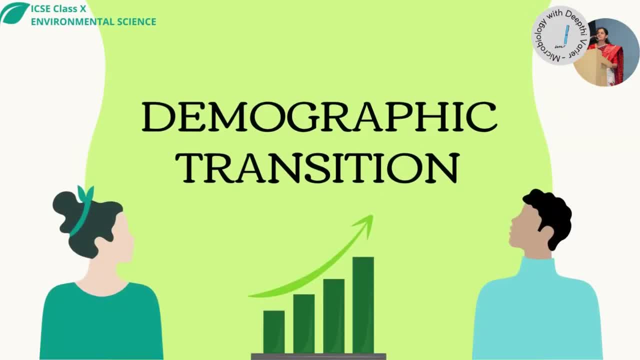 now if we see the demographic transition. demographic transition, demography as such is the statistical study of human population with reference to the size, the density of population, the distribution of population. that study is what we call as demography. and when we say demographic transition, it is the shift from the high 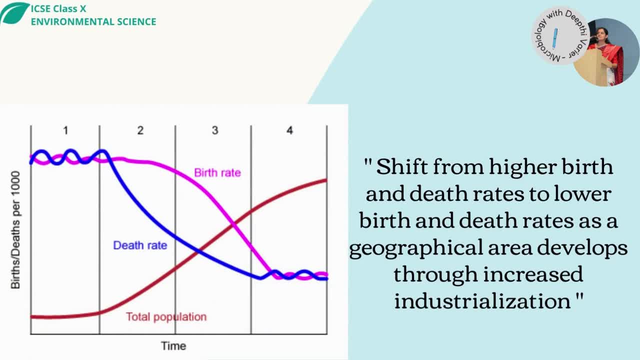 birth rate, which is seen in societies which have minimal technology or very less education or economic development, is very, very poor. from such societies, from such geographical areas, when there is a shift to a lesser birth rate- lesser, you know, lower birth rate or lower death rate, then that shift happens. that shift is what we callizada. 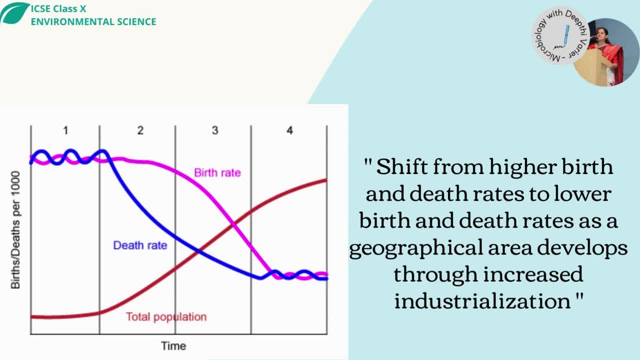 the demographic transition, and this shift mainly happens through increased industrialization. so these are what you see over here are the different stages of demographic transition. traditionally there were four stages, but now a fifth stage has also been included. now the first stage. what you see over here is where there is very high birth rate and very 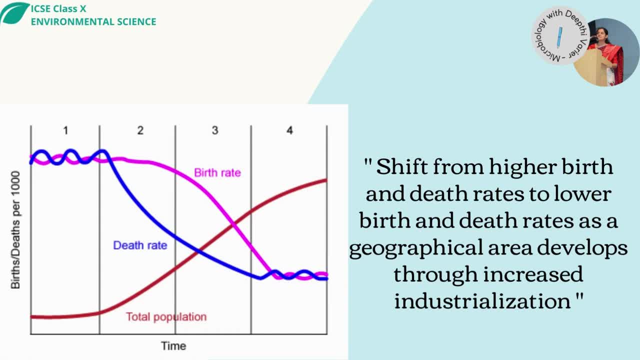 high death rate. this is mainly happening. you know, this was seen in our world until the late 18th century because the medical advancements were not so freely available to everyone. we didn't have so many medical technologies, so the birth rate also was high. the death rate also was very. 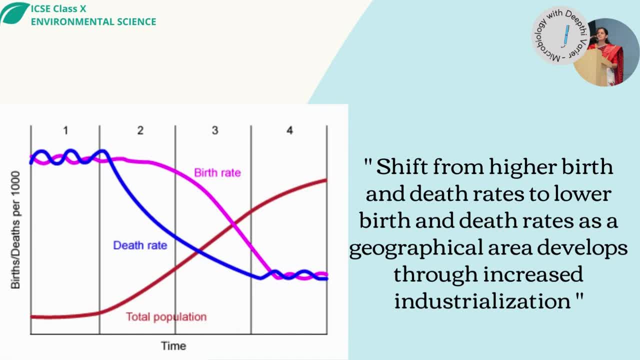 high. due to this, the population growth is very slow. that is why you can see over here the maroon colored line shows the growth of the population, because there is a lot of death also happening, even though the birth rate is very high. many children are being born. death rate also was high. 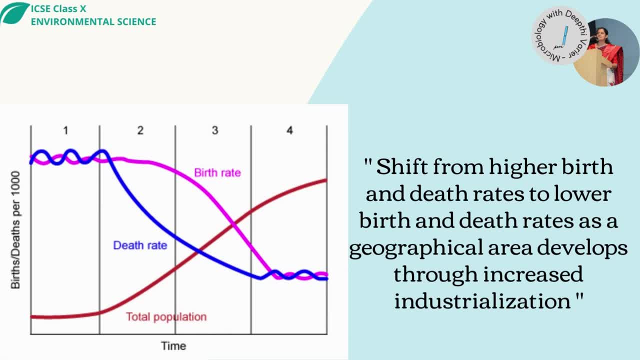 due to which the population growth is very, very slow. the next stage is where we have the death rate decreasing, but the birth rate is still high, so this mainly happens when you have health care coming in. there's more of education, food supply is better. many people get. 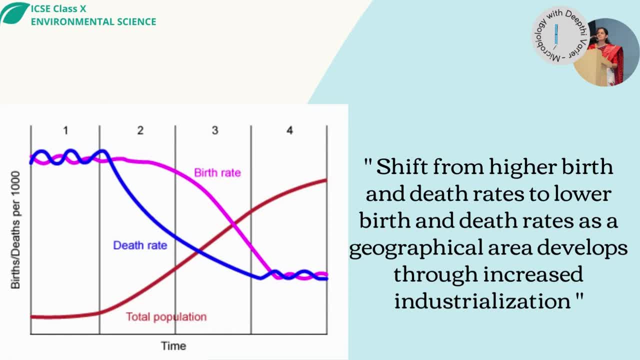 food so they don't die due to famines. this is where the death rate decreases, but the birth rate is still high. so in this stage you have population growth increasing. there's a faster population growth. stage 3 also, there is a faster population growth. growth is still increasing. it's slowly. 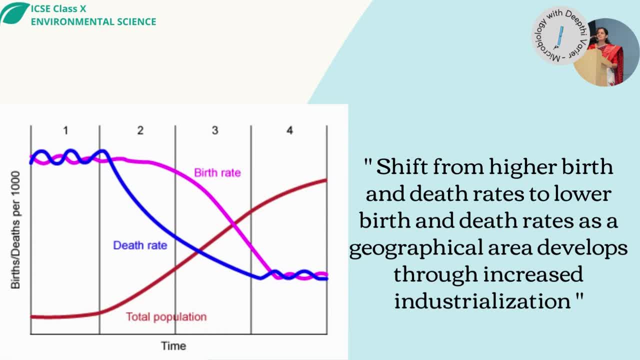 i mean towards the end end, it starts slowing down, but there is increase in the- you know- population, because the birth rate is now falling. though the death rate is low, the birth rate is also falling. this is mainly due to use of contraception or due to you know. 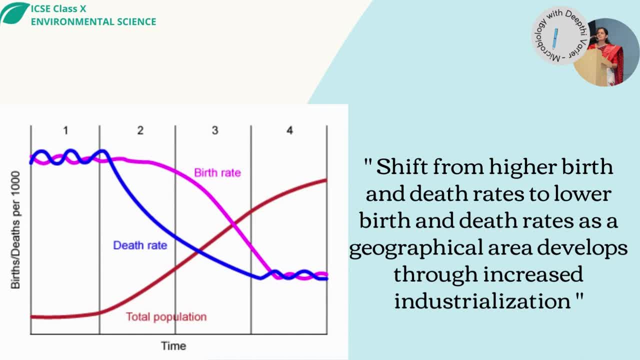 increased education, increased awareness, urbanization- women are getting educated. there are a lot of social changes that are happening. due to this, the birth rate is now falling, and fourth stage is where both are low. so the birth rate is also low. the death rate is also low. this usually 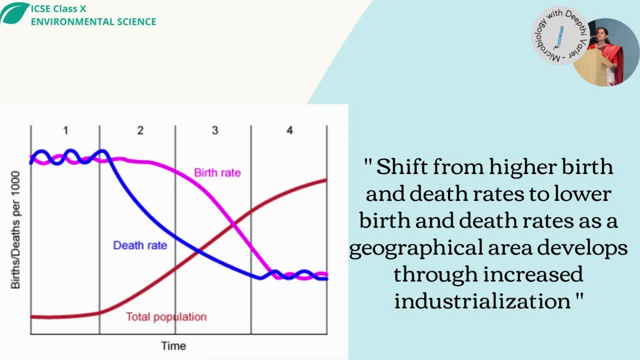 a stable population. so you can see over here the population starts to stabilize. the death rate may slightly increase after this due to lifestyle diseases or, you know, due to lack of exercise and aging population, but generally the population now becomes stabilized in the stage four. so in developed countries they have already reached stage four and in the 20th century they reached 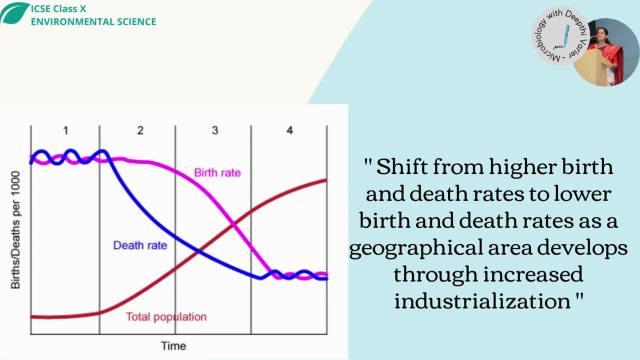 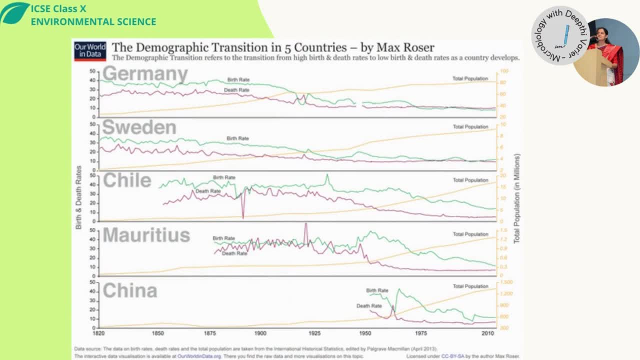 stage four, where the population is stabilized. so the birth rate is also low, the death rate is also low. let's have a look at some of the demographic transitions in some of the countries so you can see over here. this is the demographic transition of germany and sweden. as you can see the population. 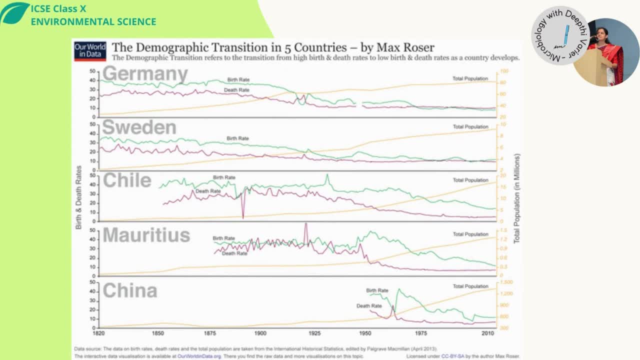 is increasing. this orange colored line is showing the increase in population. population is increasing, but the birth and death rates are pretty low, as you can see over here. you can see this in mauritius. on the other hand, though, the birth rate is still a little high, death rate is quite low. it is due to 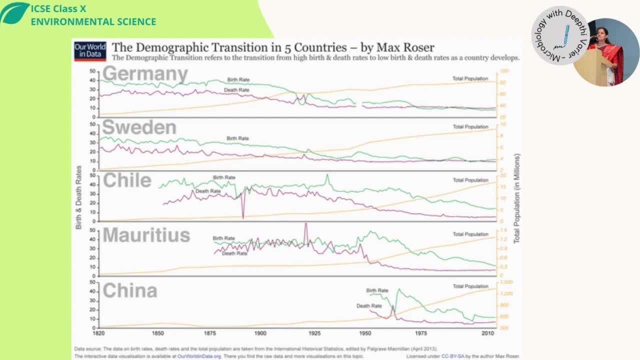 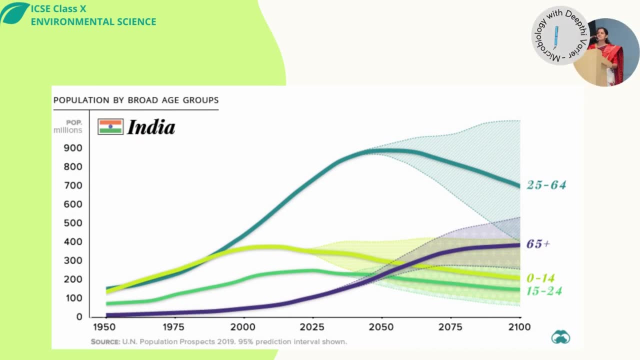 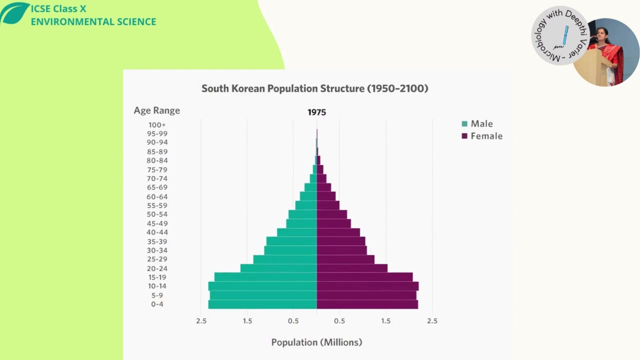 you can see china over here again. birth rate is a bit high, though the death rate has considerably decreased, but the population keeps increasing, as you can see in this graph. so this is the demographic transition of india, and what you see here is the uh, a beautiful image that is showing. 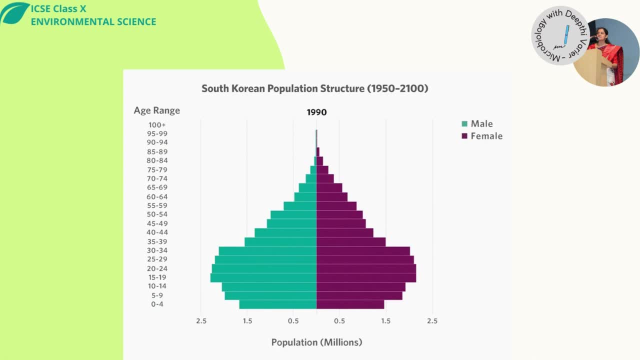 the population structure of south korea, now korea. for the first time in 2020, their population had declined and this is mainly because the fertility is very low. the fertility their fertility is rate is the lowest in the world. they have only 0.84 births per woman. what does that mean? it means 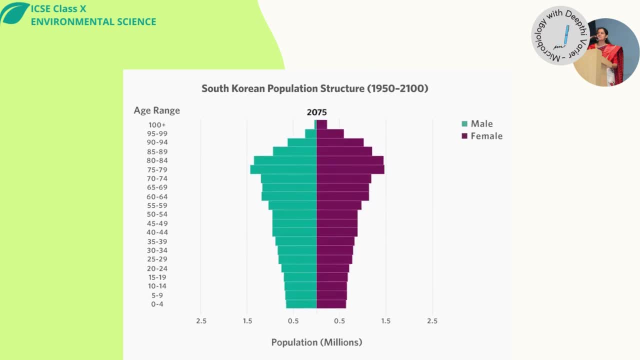 that the birth rate is very, very, very less, and that is why the population is was declining, or it was, you know, for the first time it had declined in the year 2020 and, as you can see over here, this is the prediction for the population in south korea for the next few years as well, for the 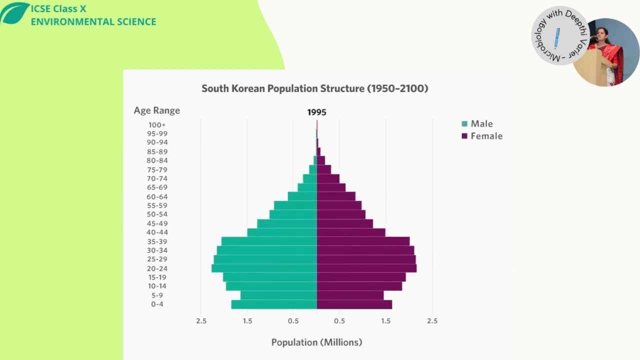 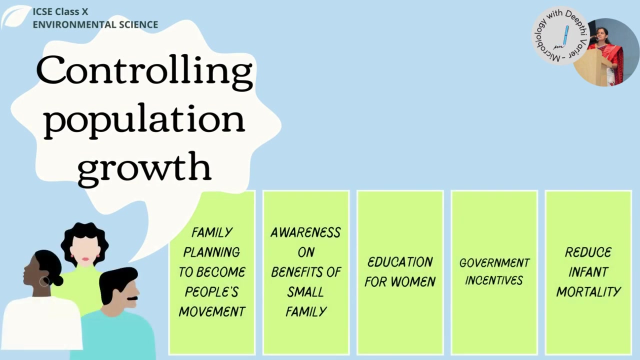 next few decades as well. so this is what the demographic transition means, that is, the shift from very high birth and death rates to very low birth and death rates due to several social changes and industrialization. now what are the different strategies that we can employ to control the 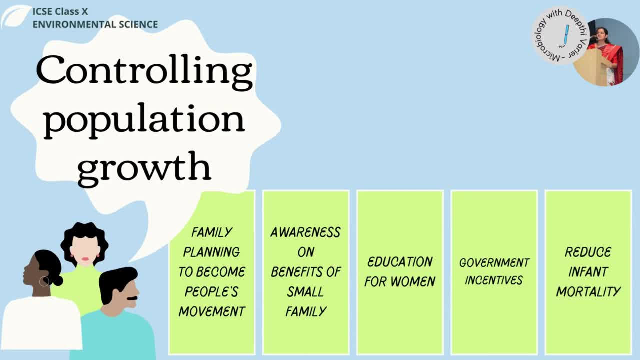 population. so, like i told you earlier, if we do not control the population, we are going to have many more changes in the climate. we are going to have a lot of- you know, a lot- more degradation of the environment than what is there already. so the strategies for controlling the population growth: 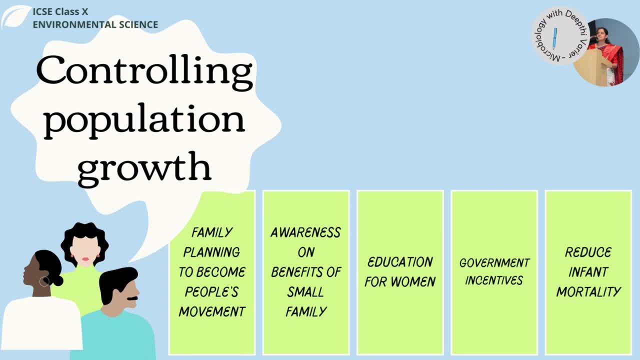 mainly in it is that the family planning or the, you know, reduction in the number of children or the birth rate reduction, that has to become a people's movement. people have to be made aware. they need to be you know, they need to feel that, yes, it should be lesser. it can't be always dictated by a government it has. 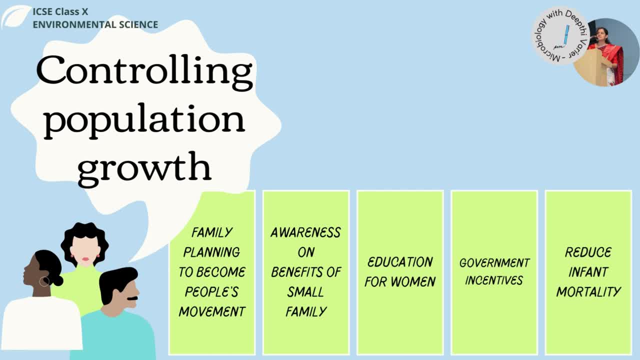 to become the people's movement. it has to become people's choice to plan their family or to have smaller families. there has to be awareness on the benefits of small family so the people should be be made aware about how the population you know is causing a lot of climate change and environmental. 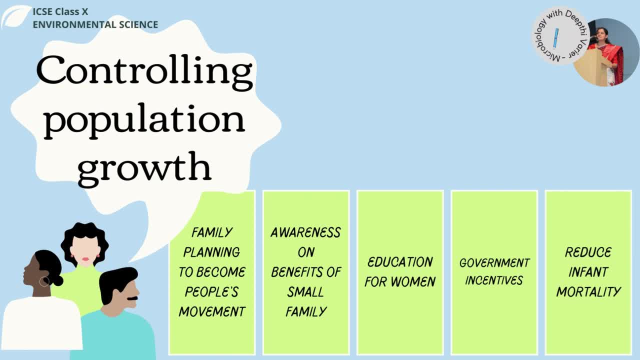 degradation and what are the benefits if you have a smaller family. and that is the reason the awareness on population is included in right from the school curriculum. so school and college curriculum does have the awareness on smaller family and what are their benefits. education for women: this is very, very important. so women-centered human development is extremely important. the women 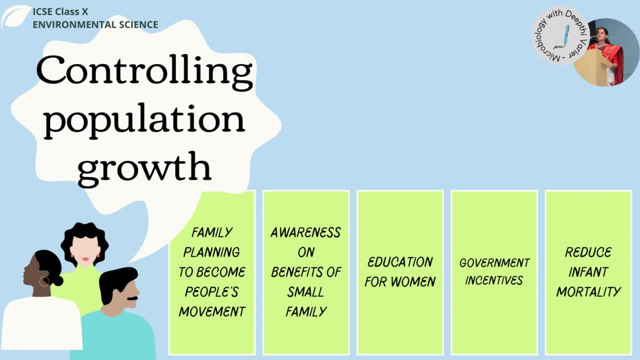 should be, you know. their education should be improved, their knowledge should be increased on the health choices that they have. they they should be made more aware about their reproductive health. empowering of women will make sure that, you know. their decision making is increasing. they are able to take decisions in their families, in their societies, and it will reduce a lot of gender-based. 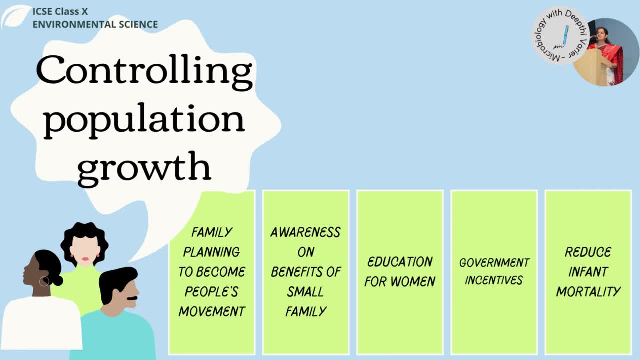 violence or gender-based discrimination, domestic violence. that can be achieved if we go for more education of women. you government incentives need to be in place. this is already there in many of the countries where government will provide facilities for employees, you know, with two children, and so if they have more. 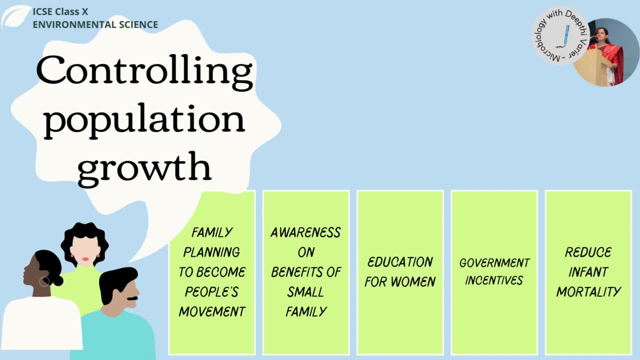 than two children, the facilities come down, due to which these incentives will motivate people to go for smaller families. contraceptives which are to be used for the birth control. they are also distributed freely amongst, you know, areas which have high population, so such kind of incentives need to be taken up by the government immediately in areas where there is a lot of gender. discrimination, and so this is one of the reasons why we are talking about this, and immediately in areas where there is increasing population growth and finally reducing the infant mortality. this is because parents, you know, should not have larger families or larger family size. they shouldn't increase the family size just so that at least a few survive. so in many countries, what happens is that the health care system is so poor, the sanitation facilities are so, you know, in such a bad condition that parents usually have many children, so that at least a few survive till adulthood. 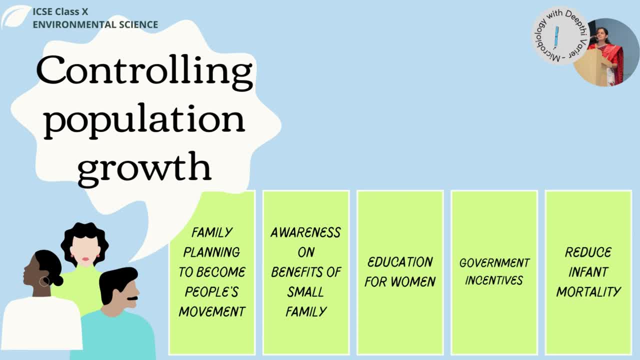 That shouldn't happen. If you reduce the infant mortality, if you ensure that the, you know, healthcare and sanitation is in good condition, then parents will have smaller families and all the children will progress to adulthood. So these are some of the strategies for controlling the 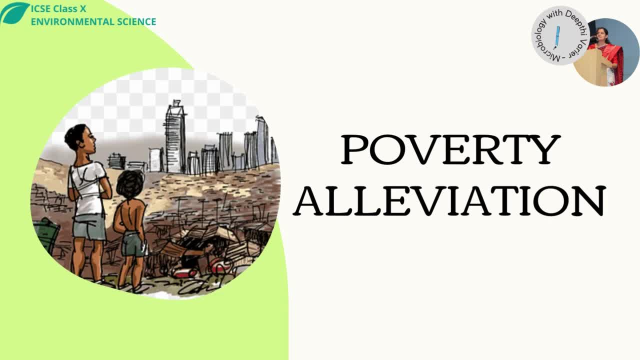 population growth. Now, when we look at poverty alleviation, this is also part of population growth, Because when we have too many people living in a particular area or in a particular country, automatically their economic status comes down. Many of them tend to be from the 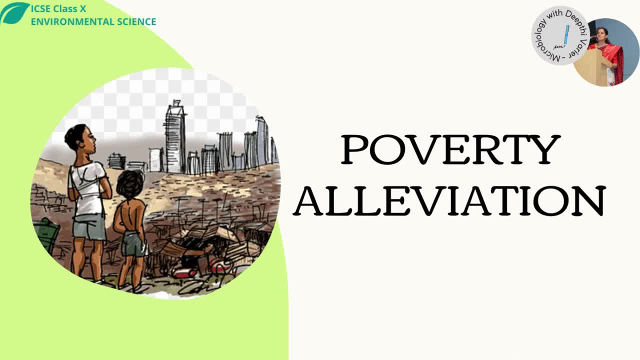 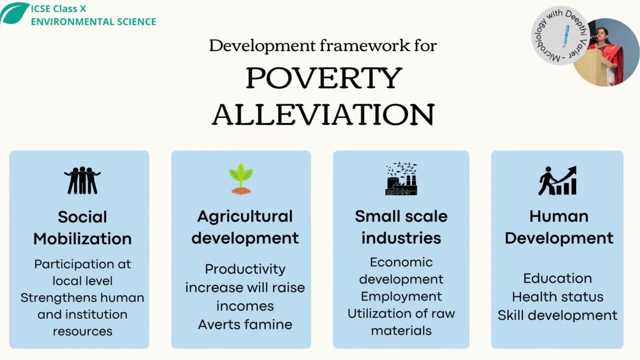 poorer sections, And that again leads to a lot of different types of problems. So we need to make sure that there are different strategies, different frameworks that are provided to reduce poverty or to alleviate poverty. The first one is social mobilization. Social mobilization- 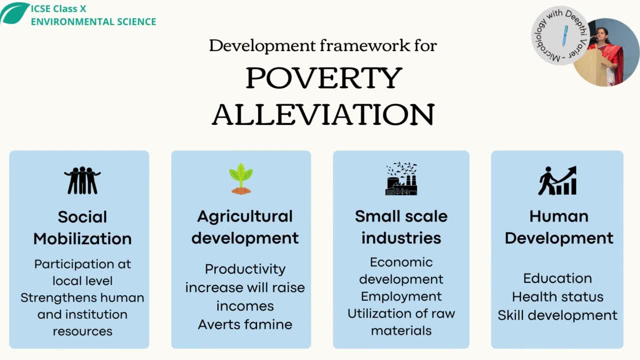 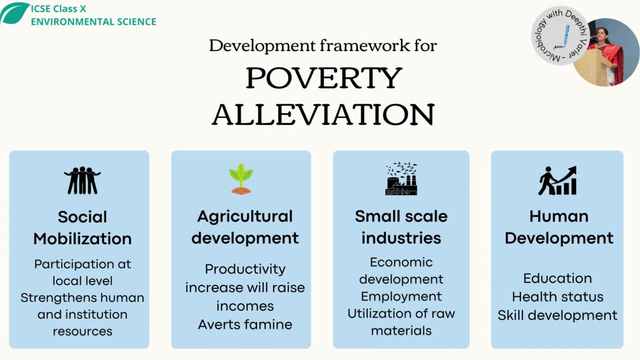 they didn't have enough sanitation facilities, So a series of awareness programs and meetings were conducted regarding basic sanitation facilities And each family. it was decided that each family would put in 20% of the work, whereas the village panchayat would do the rest. 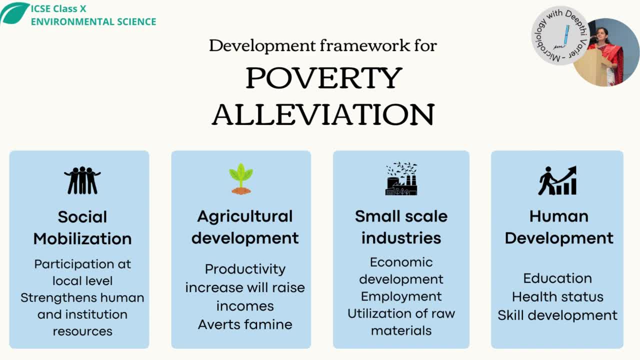 80%. But it so happened that within three months all the work was completed And, in fact, the panchayat was able to save a lot of money, because the families took it upon themselves to build the toilets and to build the sanitation facilities. So 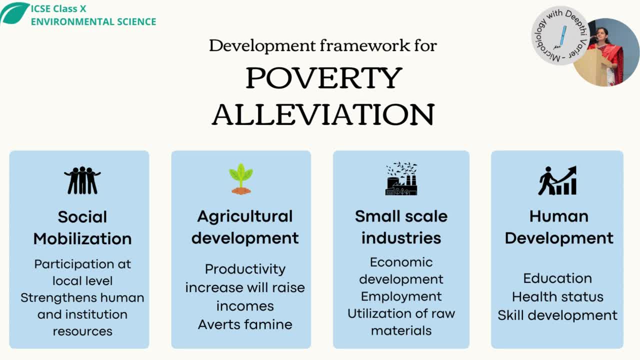 mobilizing the people, making sure that there is participation at the local level, empowering them or, you know, strengthening the human and the institutional resources at the local level, is very, very important. This helps in participation of the rural poor also. they are able to take decisions regarding themselves. it increases their access to. 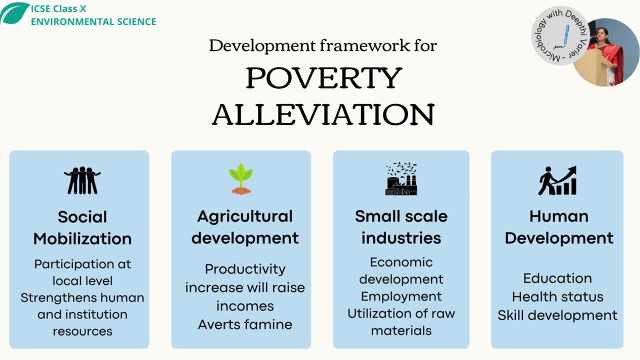 social services to production services and it also helps in making efficient use of, you know, local financial resources. So participation by the people for themselves is very, very important. That is called a social mobilization And this is very powerful in 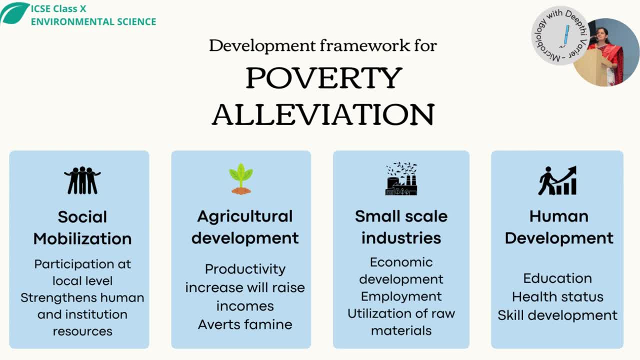 decentralization of power as well. The second method, or the second, you know strategy, is by agricultural development. When the agricultural productivity increases, automatically income will increase, And when the income will increase for the poor farmers, it will ensure that they don't.